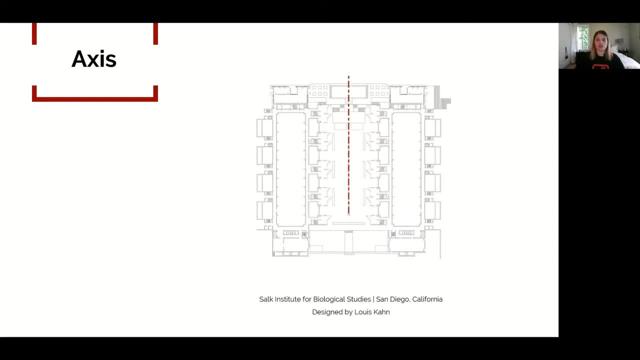 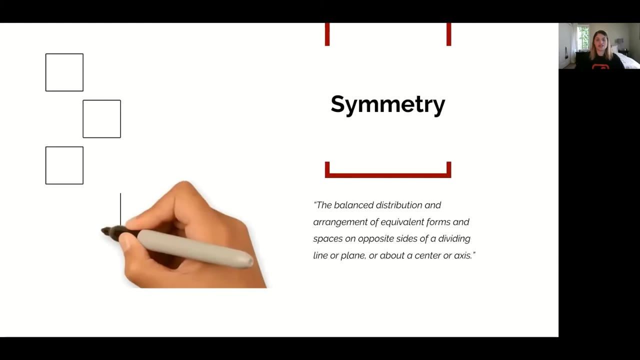 consists of a two mirror image structures with a central plaza. a thin channel of water bisects the plaza, drawing your eye toward the blue horizon. symmetry is the balance, distribution and arrangement of equivalent forms and spaces on opposite sides of a dividing line or plane, or about a center or axis. 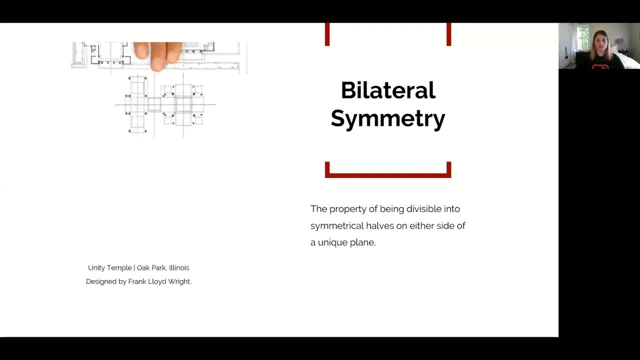 bilateral symmetry is the property of being divisible into symmetrical halves on either side of a unique plane. the floor plan of the unity temple shows multiple symmetries, both major and minor. this helps to add complexity and hierarchy to its overall composition. radial symmetry is the property of being divided into similar halves by passing a plane at any. 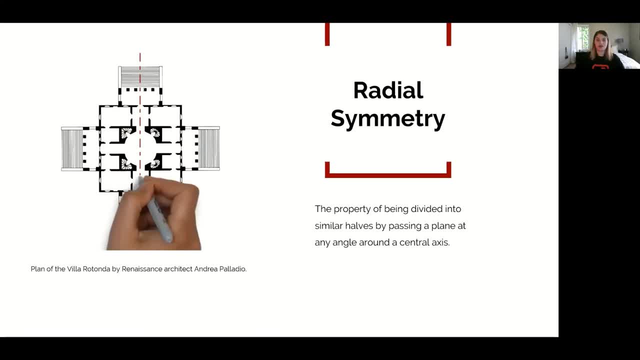 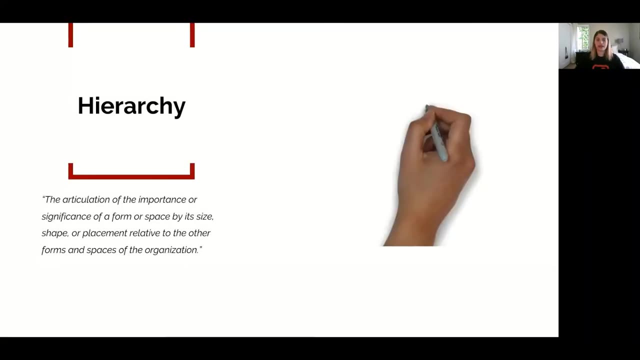 angle around a central axis. the floor plan of the villa, rotunda, as shown in the adjacent video, exemplifies this quality. hierarchy is the articulation of the importance or significance of a particular plane. it is the property of the plane in the shape of your circle. hierarchy is a form or space, of a form or space by its size. 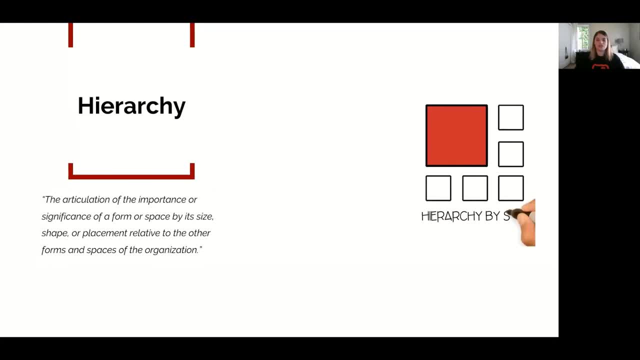 shape or placement relative to the other forms and spaces of the organization. hierarchy is often established through use of size. shape and replacement create visual significance. The red circle is made unique, contrasting with the other squares. And lastly, hierarchy by placement is achieved when a form is strategically 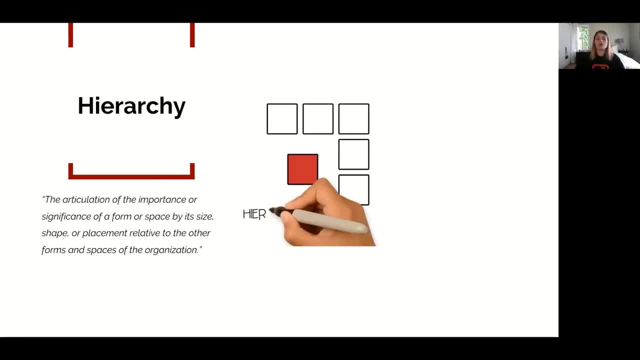 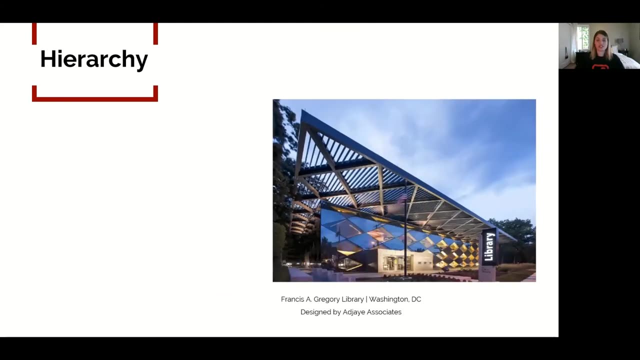 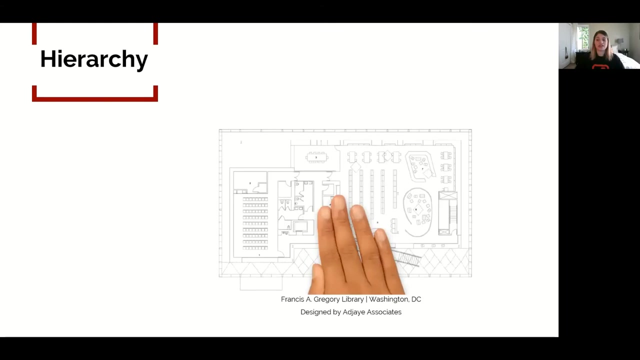 placed to call attention to itself as the most important element in a composition. Hierarchy is established on the facade of this library through differing sizes of transparent openings. The entrance is made apparent by a smaller rectangular form, more appropriate to human scale. Additionally, the floor plan of the library establishes a set of unique 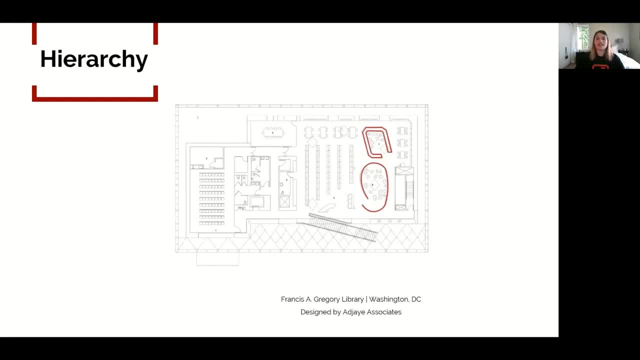 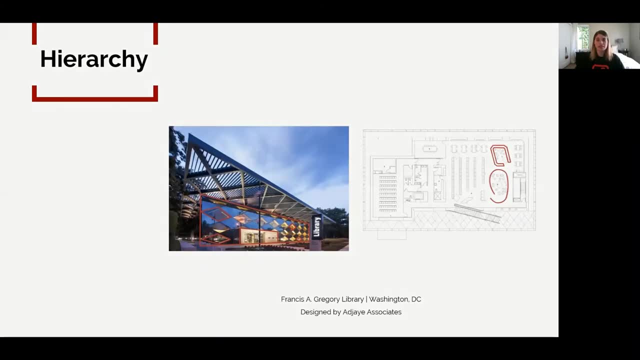 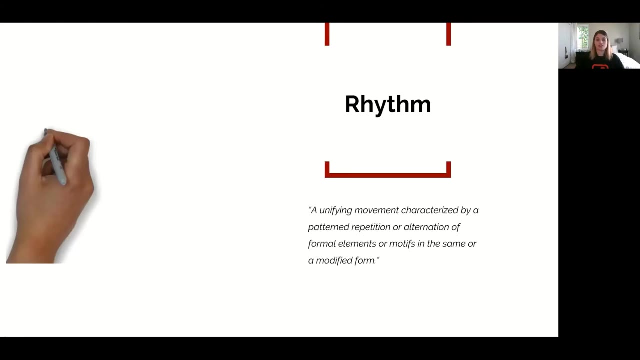 spaces by introducing forms, as highlighted by the red marker, which differs from the overall rectangular space. Rhythm is a unifying movement characterized by a pattern, repetition or alternation of formal elements or motifs in the same or a modified form. It inherently incorporates the notion of repetition as a device to organize forms and 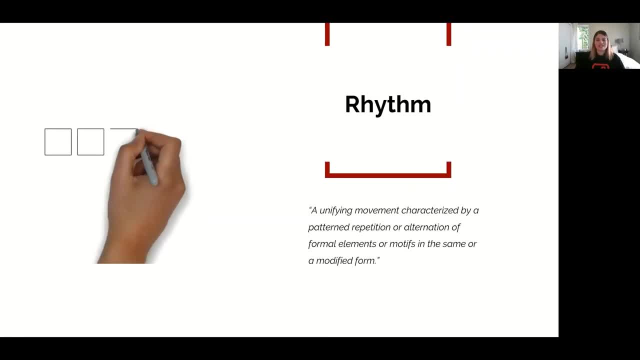 spaces. in architecture, Repetition in its simplest form can be characterized as a linear pattern of redundant elements. This is seen in the first grouping of squares which are of similar size and similar spacing. In Architecture, we may take simple repetition groupings. 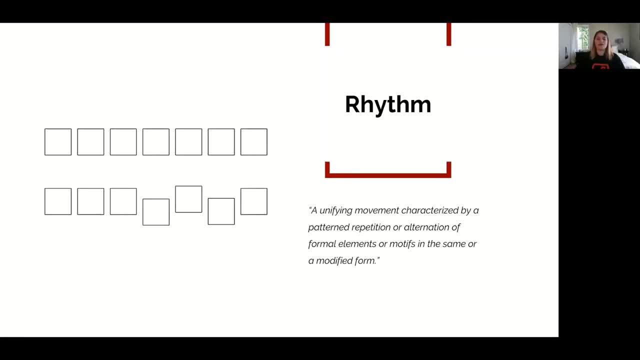 and begin to introduce slight alterations that may not be perfectly identical but still share a common trait. This is seen in the second grouping of squares, which may integraate a particular plane of space, which is similar spaces to the selection of squares on the PDF. 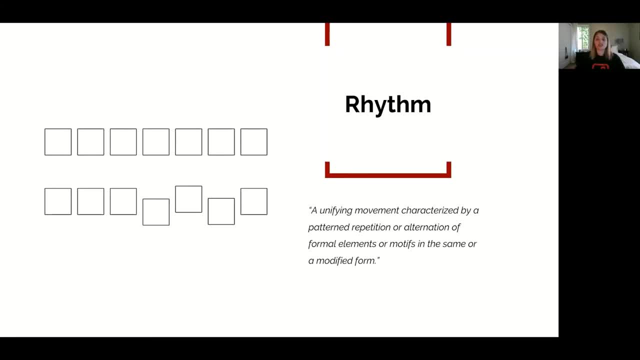 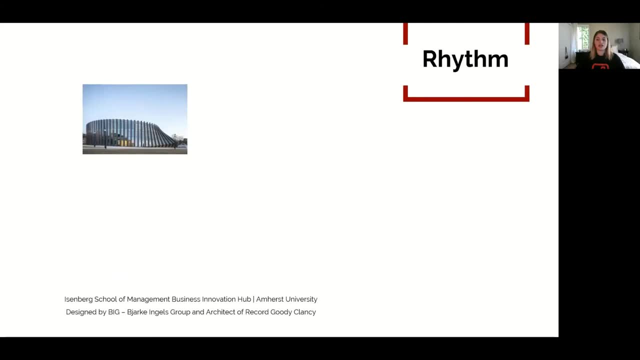 begin to shift up and down along an axis but still share similar spacing. To get a better understanding of rhythm, let's examine the Isenberg School of Management Business Innovation Hub in Amherst University. Rhythm is introduced to the building using repeating vertical elements. As we move from the back to the front of the building, the vertical elements begin. 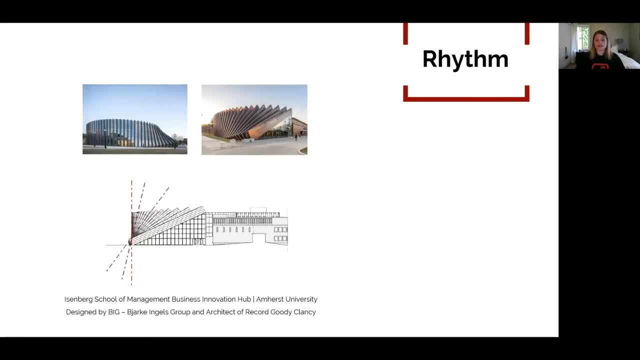 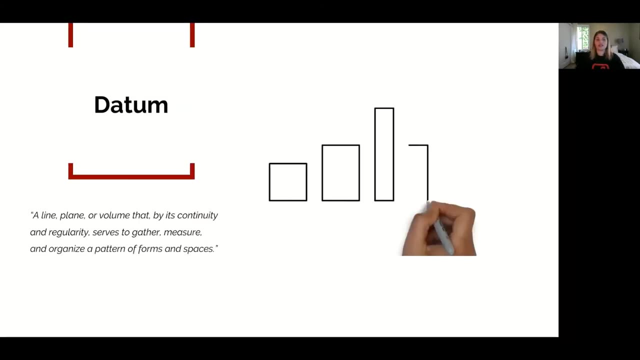 to slightly rotate about a central axis. These slight alterations may not be identical, but they still share the same vertical element and similar spacing. Datum is a line, plane or volume that, by its continuity and regularity, serves to gather, measure and organize a pattern of forms and spaces. 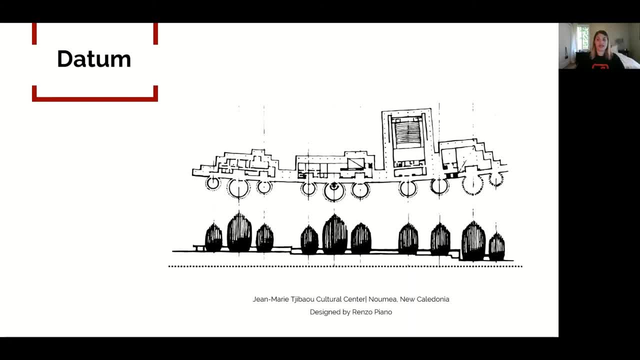 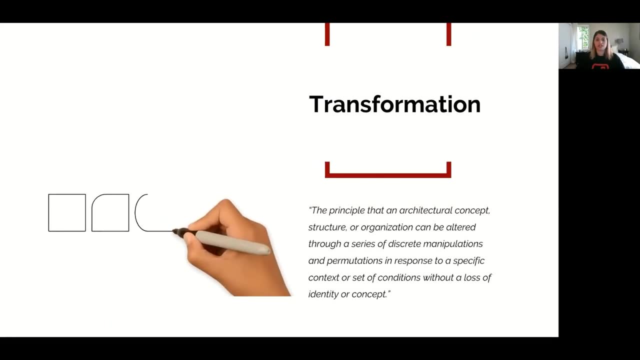 As shown in the floor plan of this cultural center, a datum is established through a common edge unifying the series of circular clusters and the small pavilions along its length. Transformation is the principle that an architectural concept, structure or organization can be altered through a series of discrete manipulations and permutations In response to a. 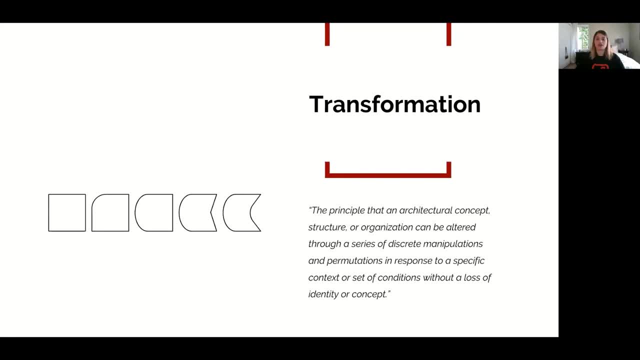 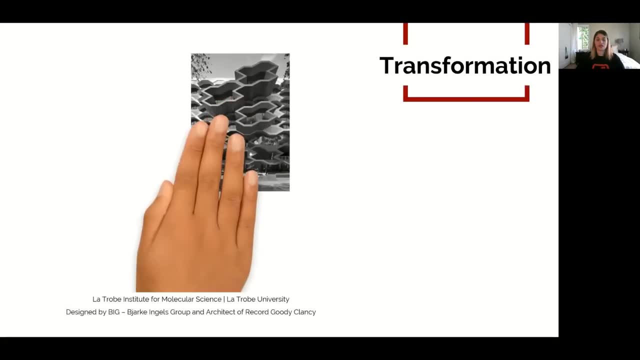 specific concept or set of conditions, without a loss of identity or concept. The facade of this building is made up of a module based on the hexagonal geometry of a molecular structure. The module transforms in size, depth, color and form, responding to the specific. 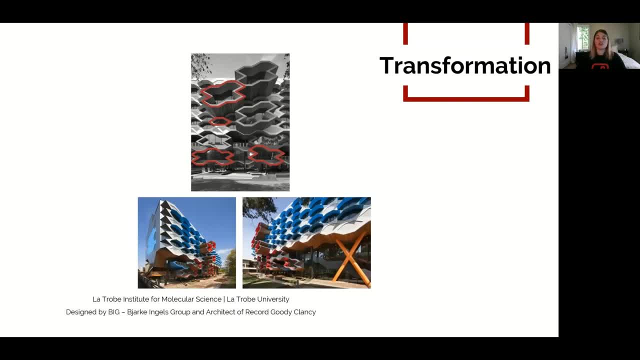 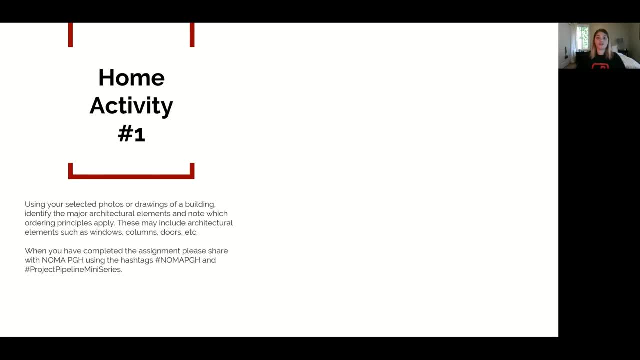 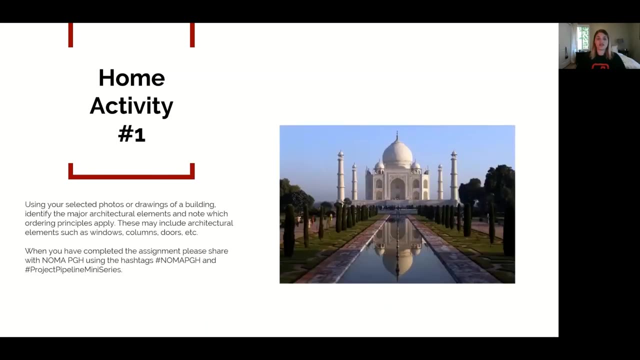 conditions and context of the design and creates a framework for several distinct styles. The building's design is designed to resemble the design of the building For the first home activity. using your selected photos or drawings of a building, identify the major architectural elements and note which ordering principles apply. 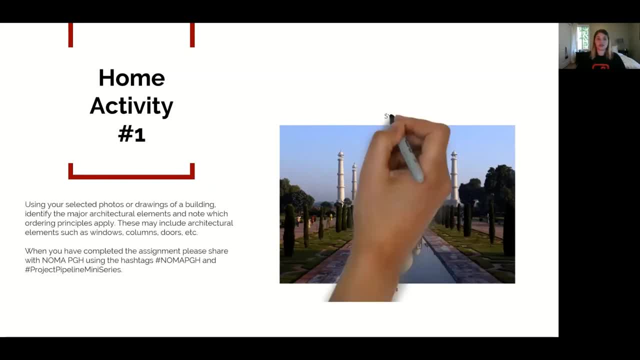 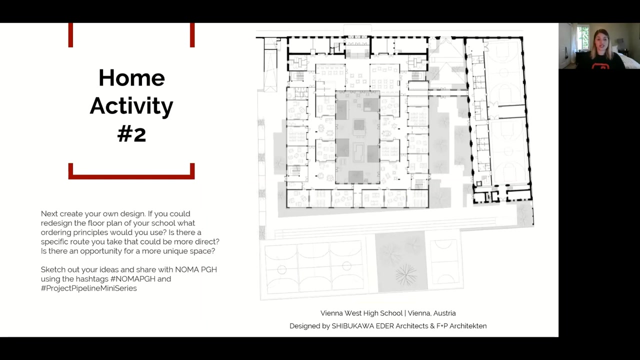 These may include architectural elements such as windows, columns, doors, etc. When you have completed the assignment, please share with NOMAPGH using the hashtags NOMAPDH and Project Pipeline. mini-series For home activity two: create your own design If you can redesign the floor plan of your school. 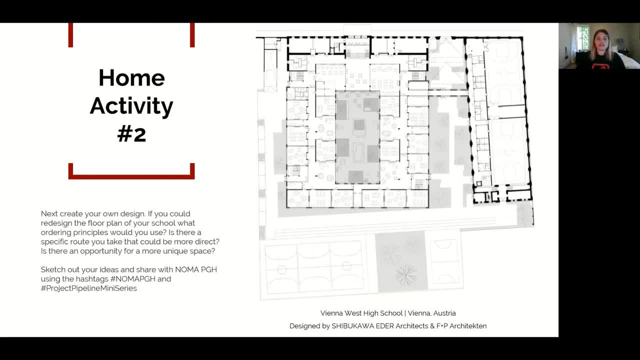 what ordering principles would you use? Is there a specific route you take that could be more direct? Is there an opportunity for a more unique space? Sketch out your ideas and share with NOMAPDH using the hashtags NOMAPDH and Project Pipeline mini-series. Thank you for participating in Project. 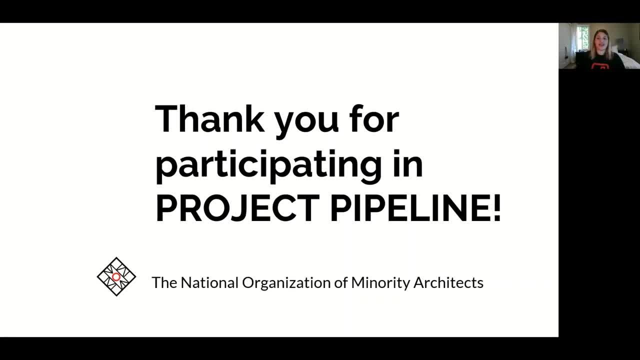 Pipeline, I hope you've enjoyed our lesson today and we look forward to seeing your work.